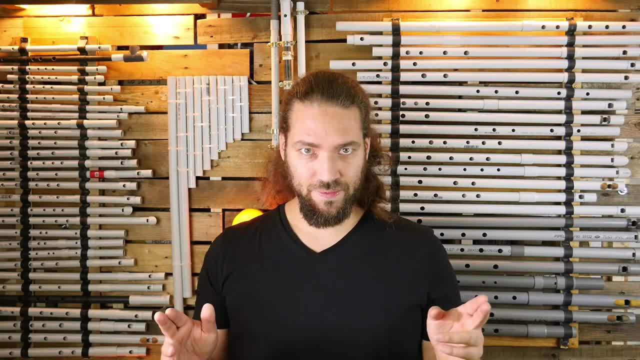 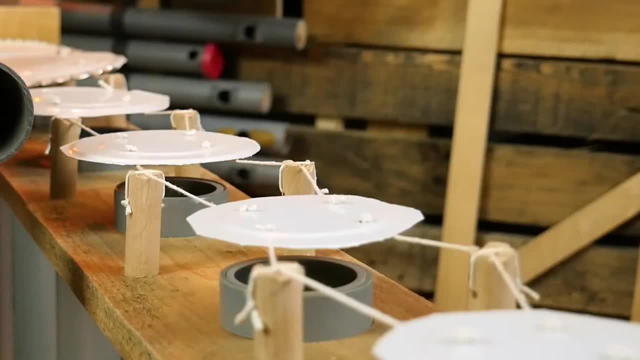 on the tin can type. Yes, there is tin can types, With or without The bump. You will have to try a lot lids to find a complete scale. You can also tune the lids by cutting the edges and put some resonators to make a gamelan. 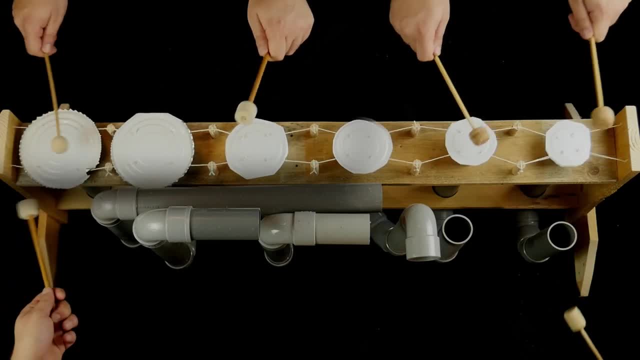 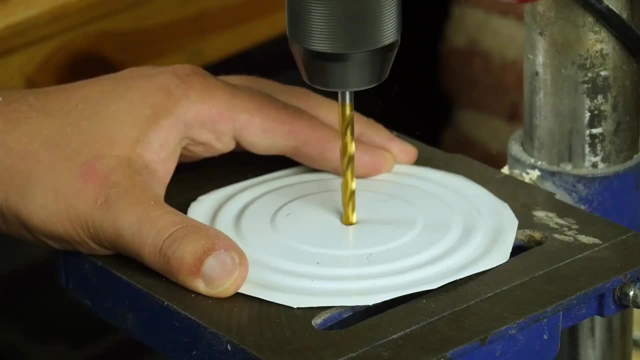 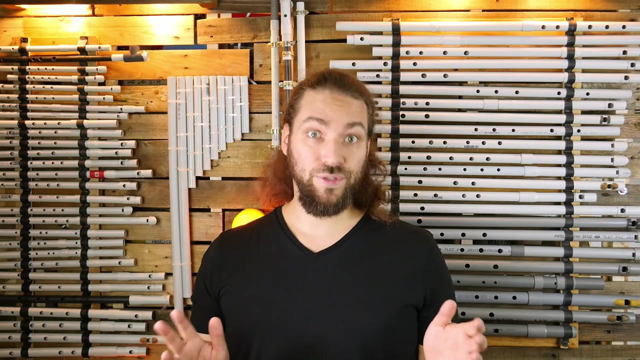 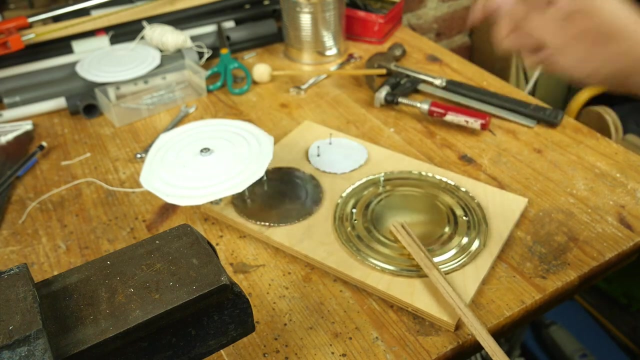 style instrument To play those like cymbals. we're going to drill in the middle and bolt it tight. Here again we have a note for each lid. With the two tunable you can make a tuned set or a cymbal added to the other sounds. 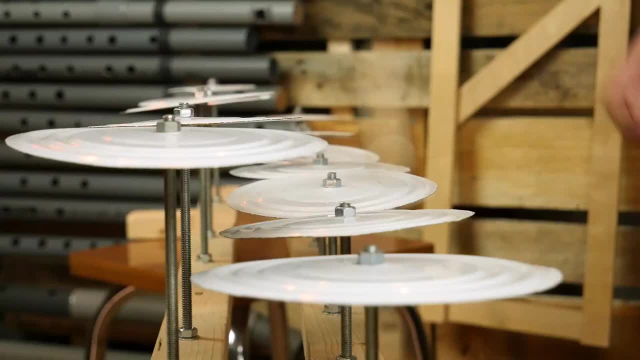 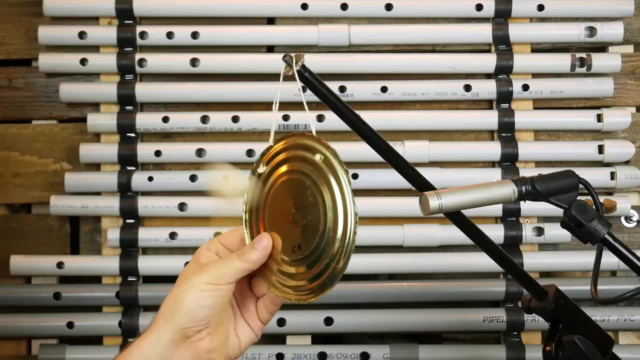 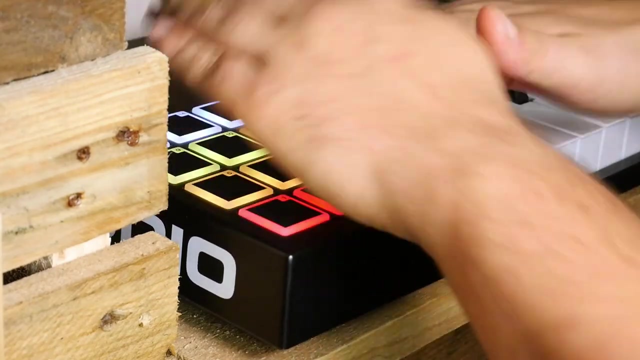 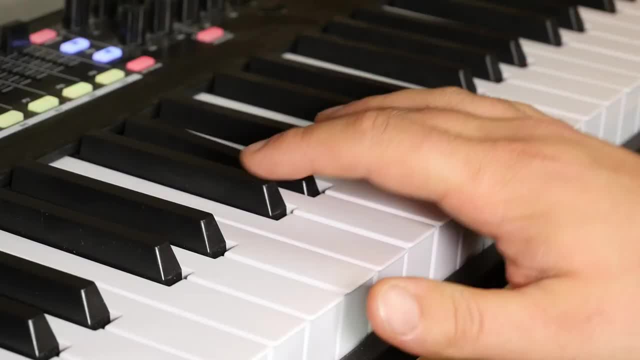 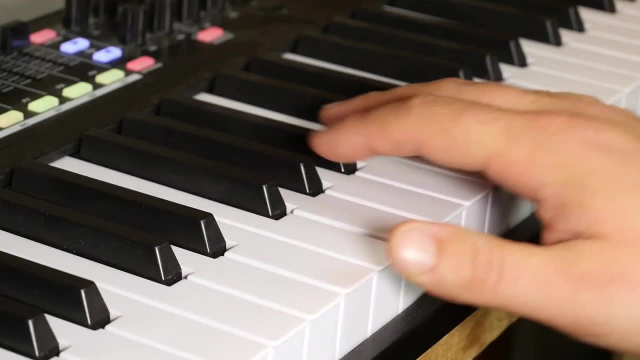 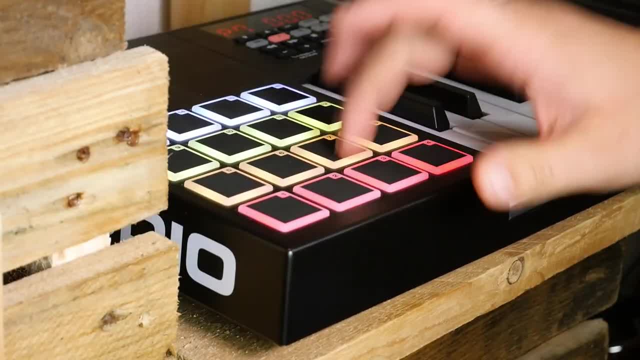 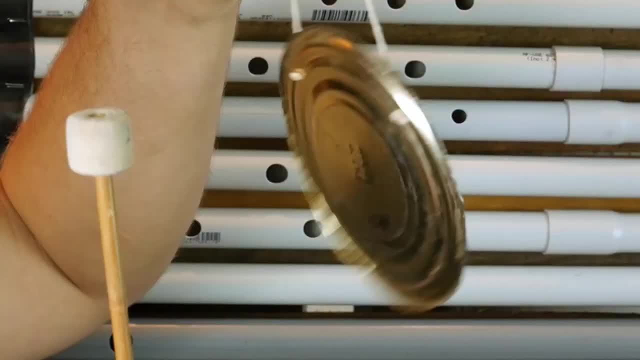 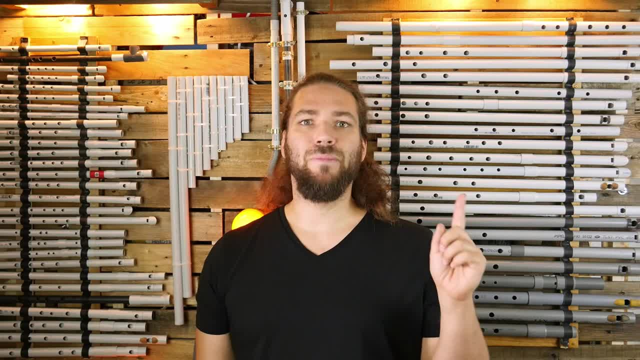 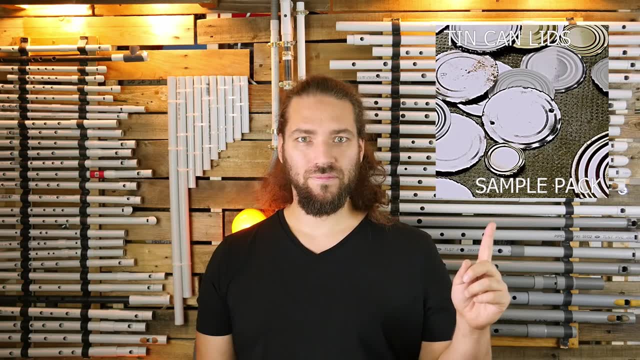 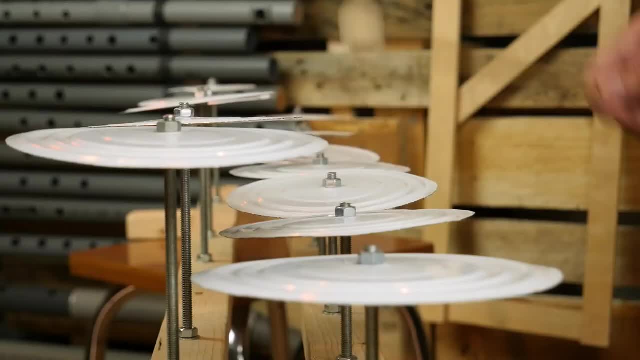 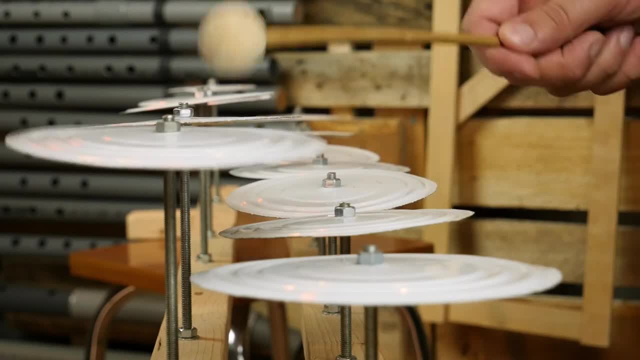